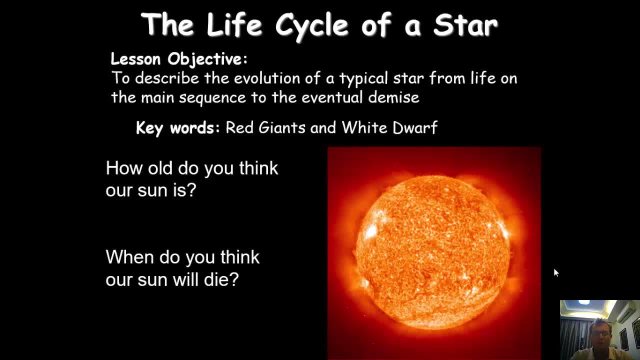 So that's a thing to think about. So, first of all, how old do you think our sun is And what do you think our sun is? How do you think our sun will die? You may know this, you may not know this. 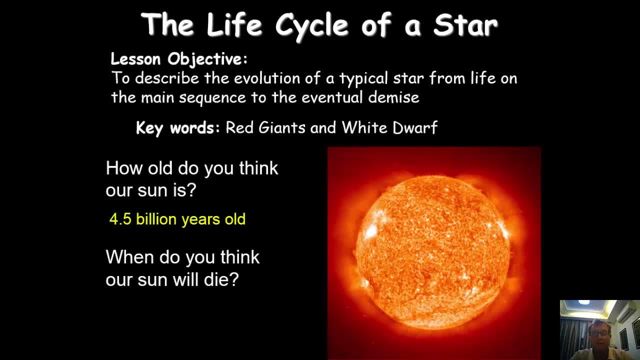 Our sun is about 4.5 billion years old. It's actually about about give or take a billion years about halfway through its life, So there's about 5.5 billion more years of typical star life ahead of it. 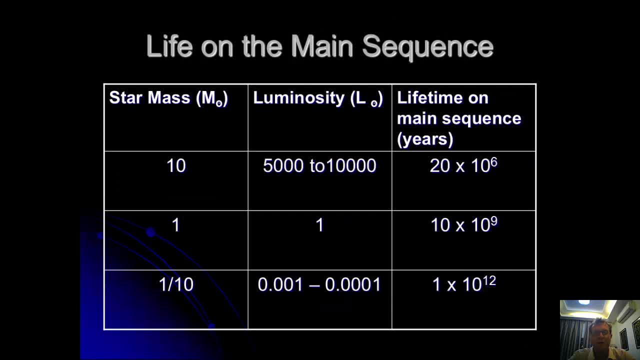 Now, all of this, as I said, is dependent on the mass. I mentioned this before. But life in the main sequence, the timeline, is very much dependent on the original mass of the star. If the mass of the star is very small, 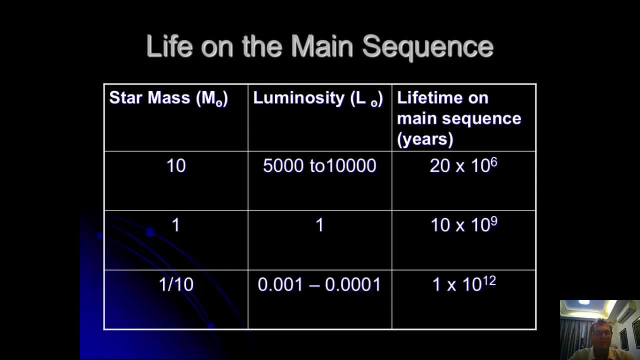 we've got one tenth of the solar mass, then what we find is that it's much less bright, but also it tends to have a much longer lifetime. on the main sequence, Whilst we use the example of a star which is ten times the mass of our sun. 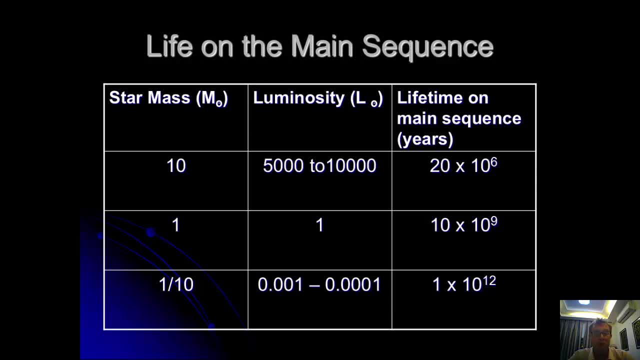 it shines much, much, much brighter, up to 10,000 times brighter. yet the lifetime of the span is only about 20 times 10 to the sixth years. So the more massive a star is, the brighter it shines, but the shorter its life. 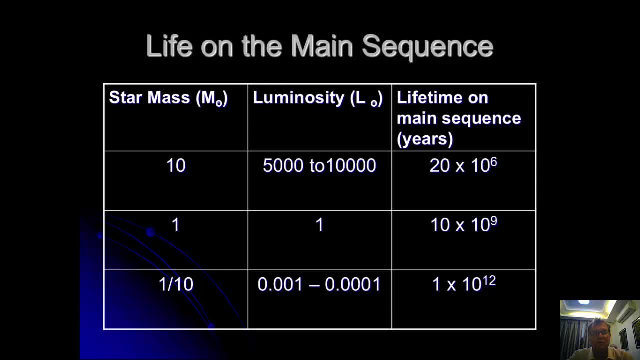 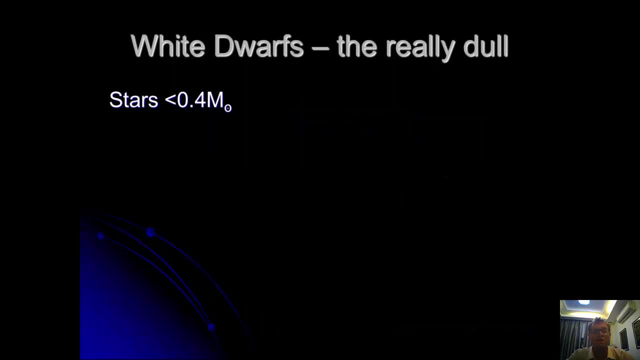 Undoubtedly, there's an analogy towards rock stars today there. So let's now think about stars which are really, really small, So a star which has a mass of under 0.4, that of our sun. well, eventually the hydrogen runs out. 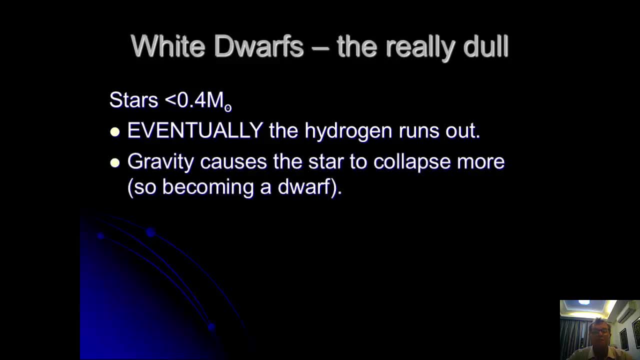 and then, once the hydrogen runs out, gravity causes the star to collapse some more, so becoming a dwarf. nothing else really happens. there's no further ignition and we have this little warm ball which cools down. for a turn It's a white dwarf and eventually that remnant heat goes away. 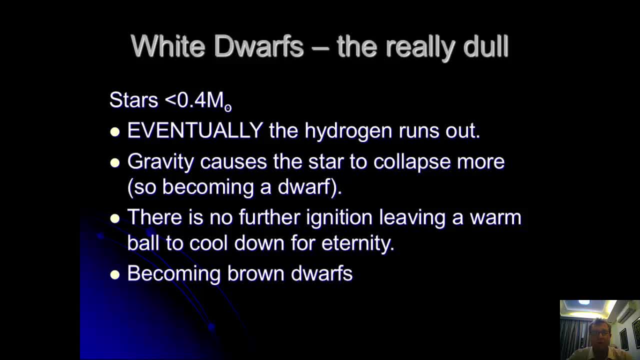 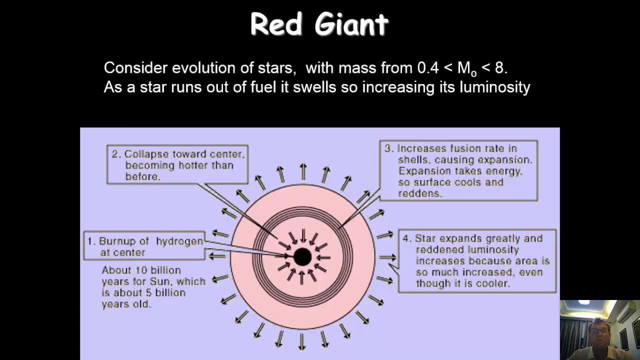 and finally becoming a dark brown dwarf. So that's for really small stars. Now for stars which are a bit bigger, with masses from 0.4 to about eight times that of our sun. as the star runs out, it swells, so increasing its luminosity. 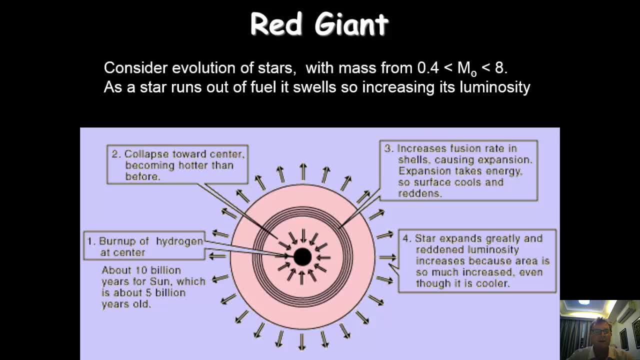 becoming what's known as a red giant. Now how this happens is we have the burn up of hydrogen at the centre. that means there's a collapse towards the centre, so that becomes hotter than before. This in turn increases the fusion rate in the shells outside. 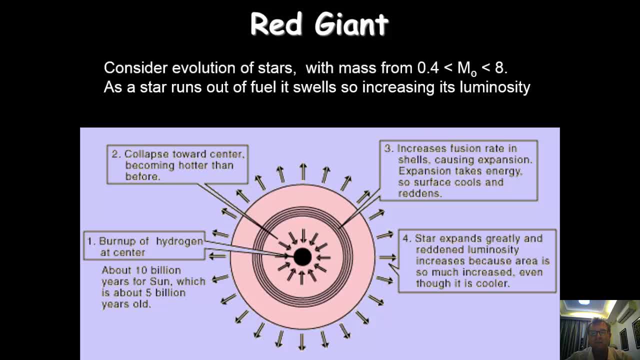 and that causes them to expand. but this expansion at the same time spreads the heat out and causes the surface to cool. So the star expands greatly and the red in luminosity increases because the air is even more increased, even though it's cooler. 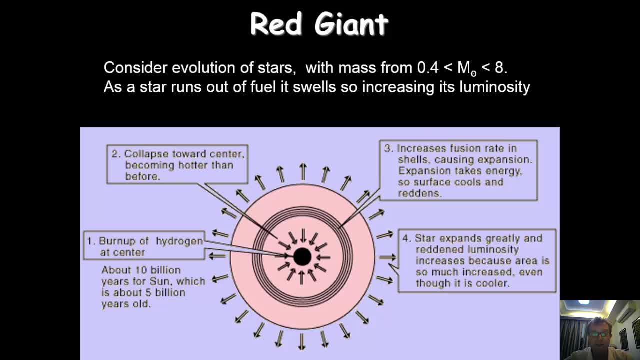 And this is what's going to happen to our sun at some stage. So our sun is going to become a red giant and when it does this, the red giant process is going to envelop planet Earth, And Mars is going to be as close to the surface. 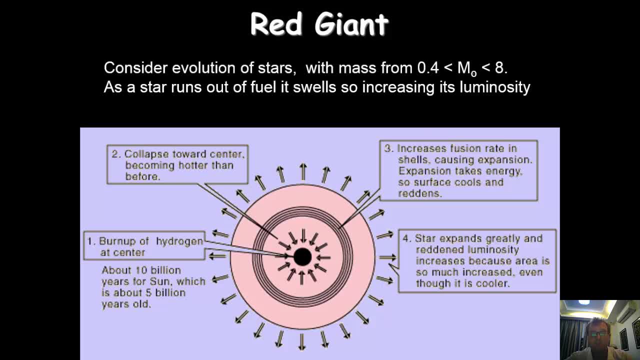 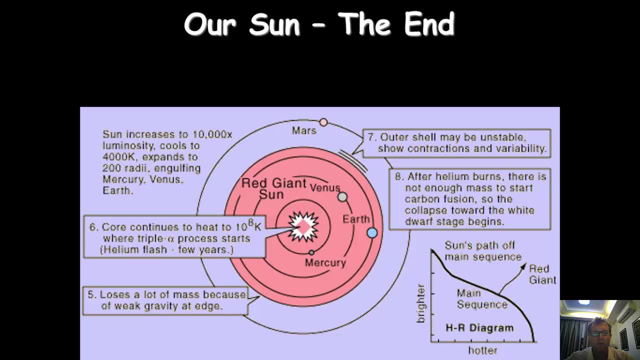 as Mercury is to our sun at this moment in time. So, as you can see what we have with our sun, we have our core continues to heat to 10, to the 8, where a triple alpha process takes place, and so that's known as a helium flash. 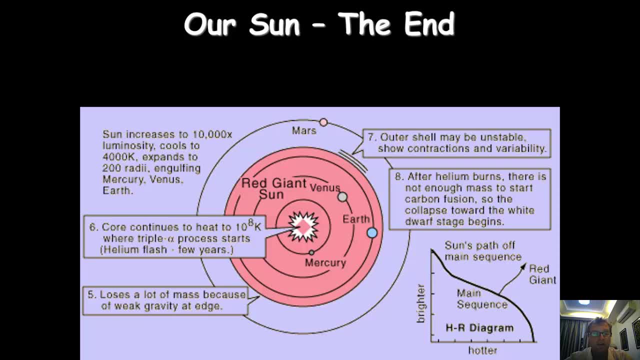 so helium is produced, It loses a lot of mass because of a weak gravity at the edge, so it's often outer. shells become often quite unstable due to the contractions and variability, And after the helium burns there's not enough mass to start anything more. 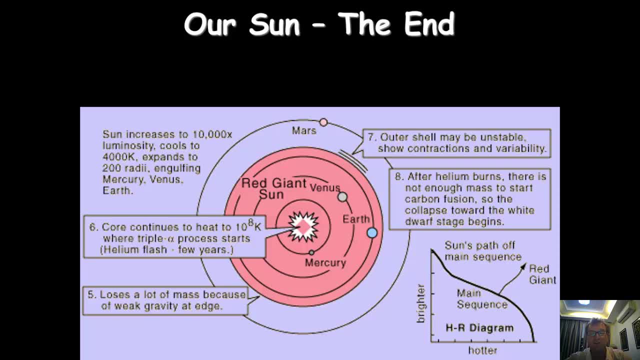 so after that it becomes a red giant and then just slowly contracts and collapses to become a white dwarf. It does have a main sequence path. so for the main sequence: it goes up towards being a red giant and then cools back down and drops down. 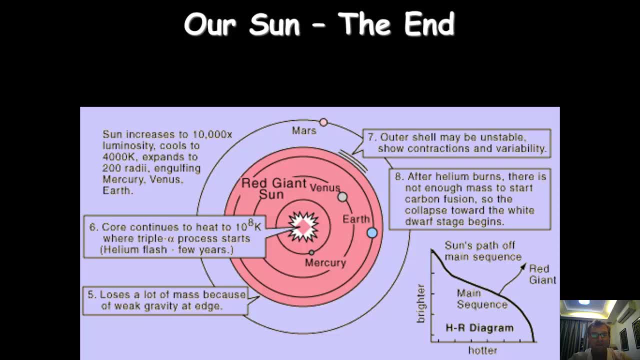 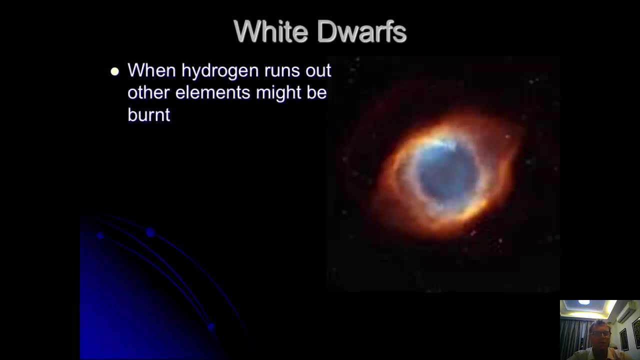 to being a white dwarf. So there's a passageway there And these white dwarfs. so when the hydrogen runs out, all of the elements may be burnt. nuclear synthesis here, but at carbon, no matter what, there's, no more fusion can take place. 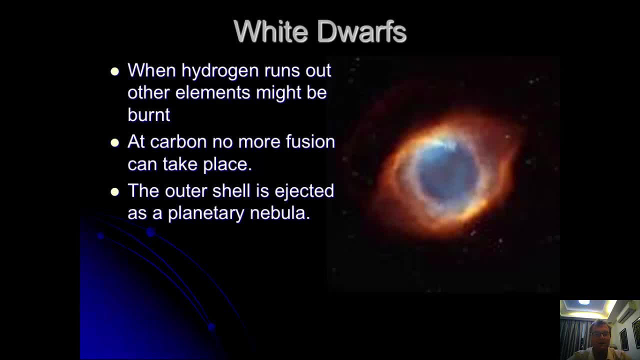 That's the end of that. So the outer shell is ejected as a planetary nebulae. So earlier on, remember, I said that those outer shells can be quite unstable, so often they can be ejected and we can see this in a 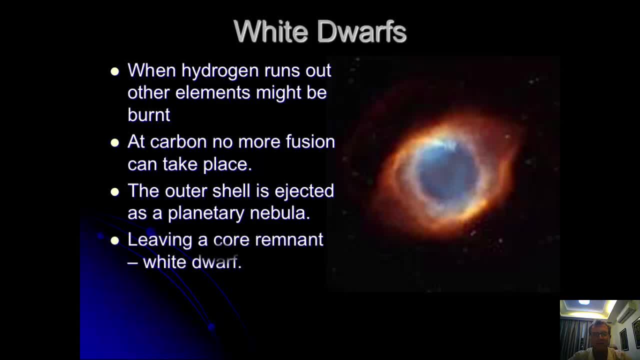 the image which I'm showing here. and the remnant, the core, becomes the white dwarf. Now note: a white dwarf cannot have a mass that is greater than 1.4 times the mass of the Sun, otherwise it becomes a neutron star. 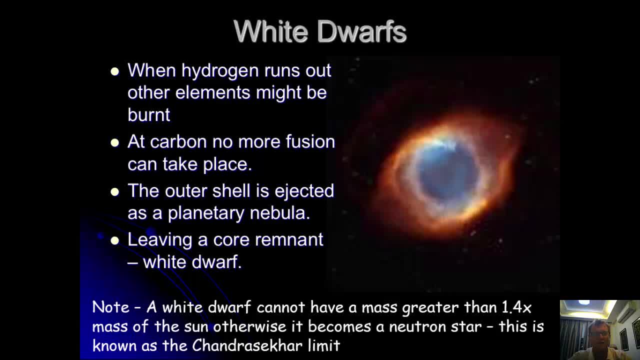 And this limit is known as the Chandrasekhar limit, and we'll explain what a neutron star is later on. but what we're saying here is that even a star which has a mass 8 times that of our Sun, it loses a lot of mass. 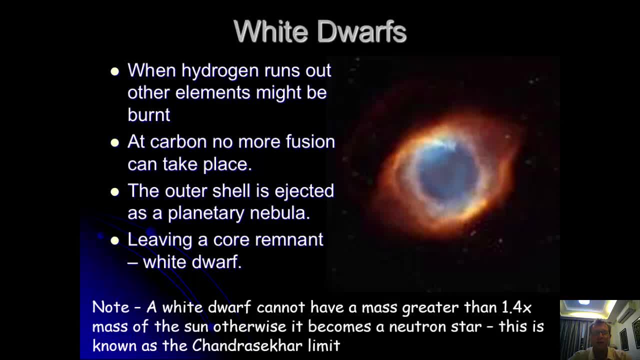 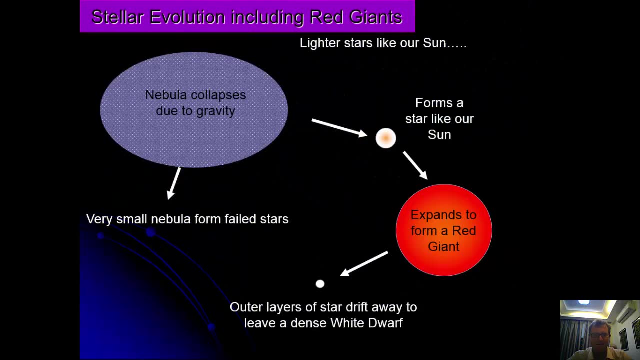 due to ejecting the outer shells, and that core remnant tends to not be very big- And I'm going to talk about what a neutron star is in another video, as it happens, but just jot down that there is a distinction there. So if we think of this in 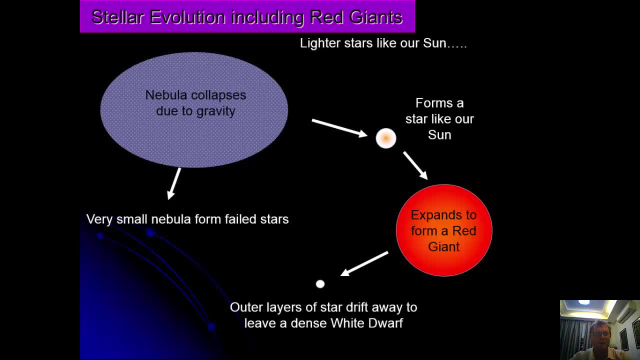 a diagram. we have a nebula, a cloud of some sort, and that collapses due to gravity and if there's enough mass there, if it's too small, we have failed stars. it will form a star like our Sun. this will expand to form a red giant. 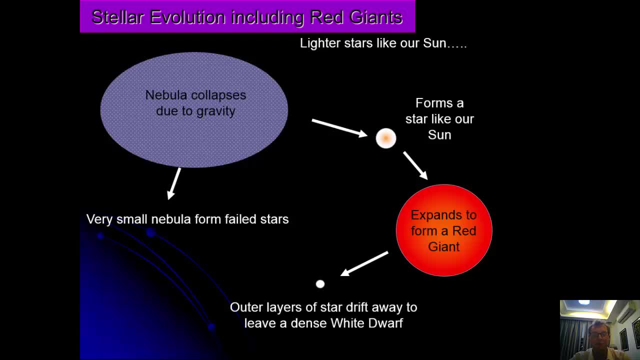 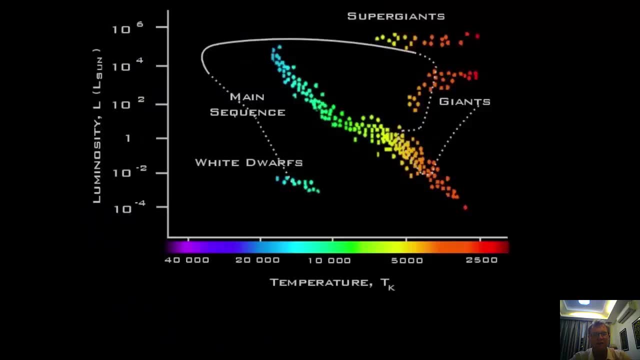 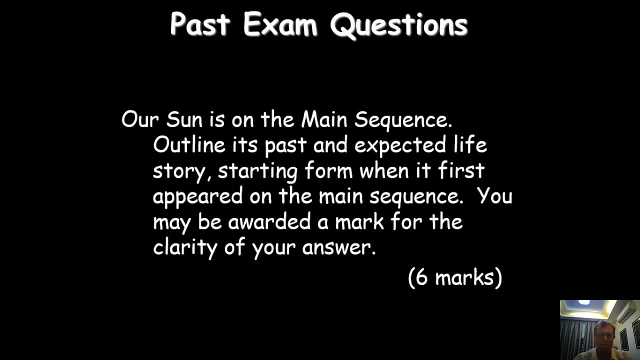 the outer layers will drift away to leave a dense white dwarf. That's the story of stars like our Sun. Now, if we tell this story by looking at the motion around the main sequence, we'll just go back to that. what we can see here is that 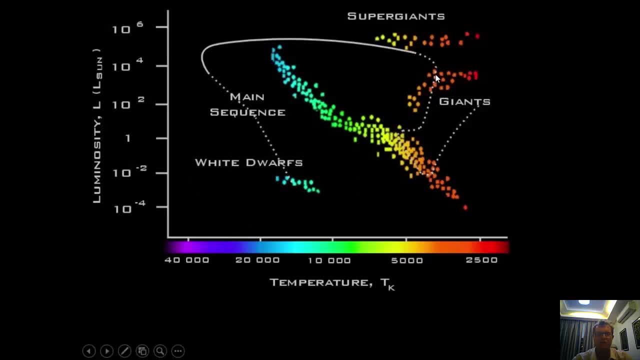 it's on the main sequence and it'll expand as a red giant and then it will just cool down and drop to being a white dwarf eventually. So that's the HR diagram story of a star much like ours. So past exam questions. 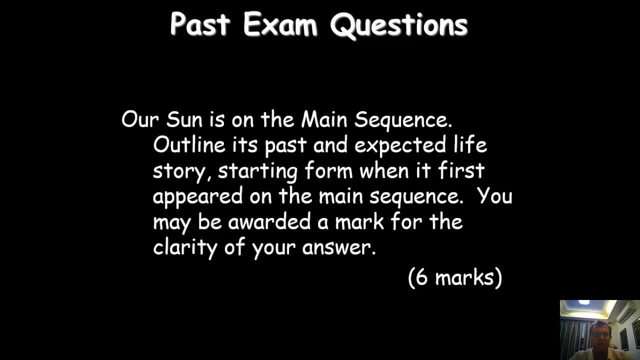 it says our Sun is on the main sequence. outline its past and expected life story starting from when it first appeared on the main sequence. You may be awarded a mark for clarity of your answer. So it's basically: can you clearly tell the story of our star? 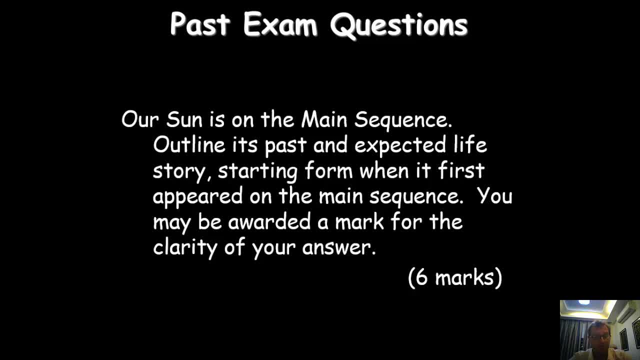 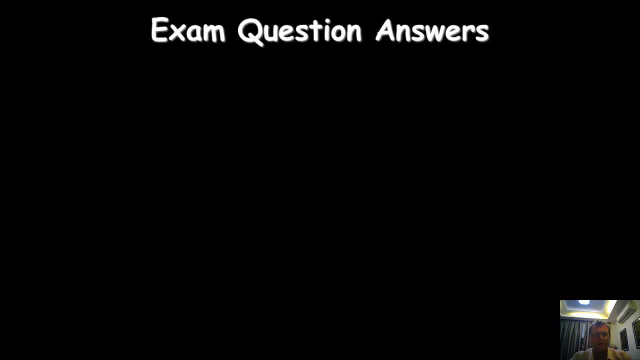 providing as much detail as possible. Take a moment, try and jot down what you can remember. what have we spoken about? And the answer would be: it gained some mass from the cloud collapse after the hydrogen ignition. So that means that, just as the star formed, 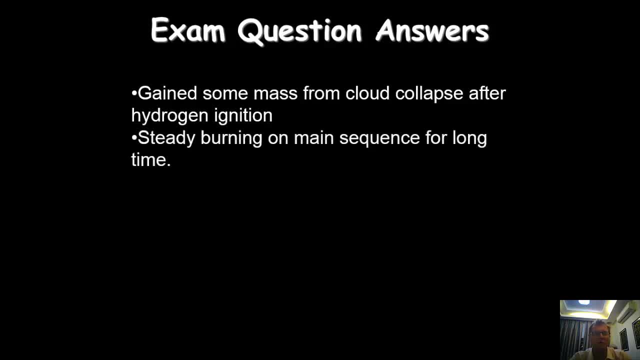 there may have been a little bit more mass falling onto it. It stays on the main sequence for a long time. As we mentioned at the beginning, this is going to be probably about 10 billion years. Then it forms a red giant With a red giant. 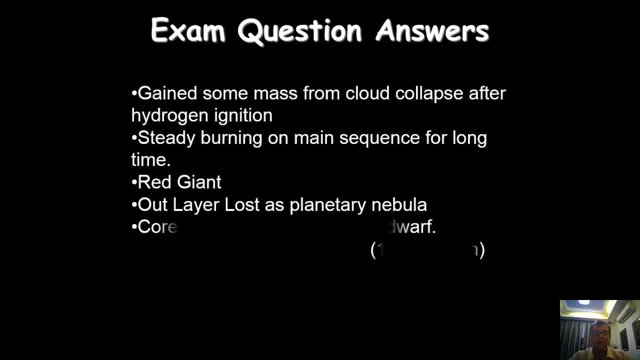 the outer layer is lost as a planetary nebulae, leaving the core remnant behind, and then it becomes a white dwarf. So that would be the story of a star much like ours And, as I've said before, a lot of the astrophysics. when we're telling stories, 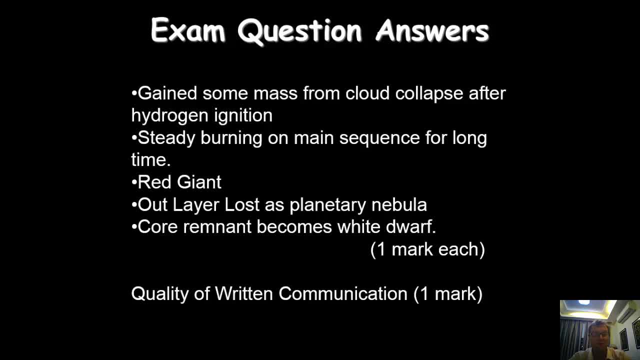 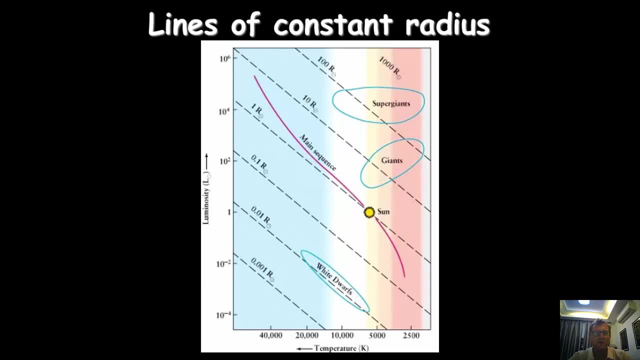 there's sometimes a mark for the quality of the written communication. A final note: here we have what's known as the lines of constant radius, And what we can see here is that we find, if we go across the main sequence, there's these lines. 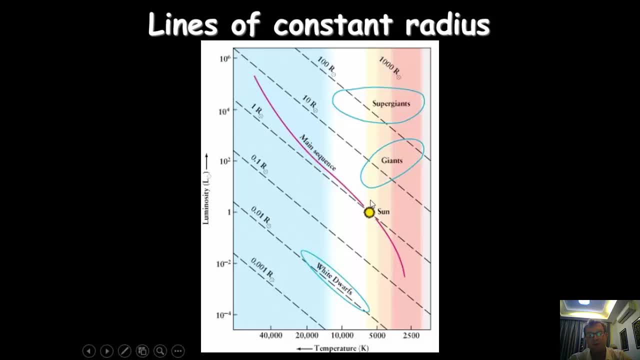 and these lines really describe stars of a similar radius. So we can see here that even though there's some stars which potentially could have a greater luminosity, they may have a similar radius as our Sun because they're a little bit more tightly bound.